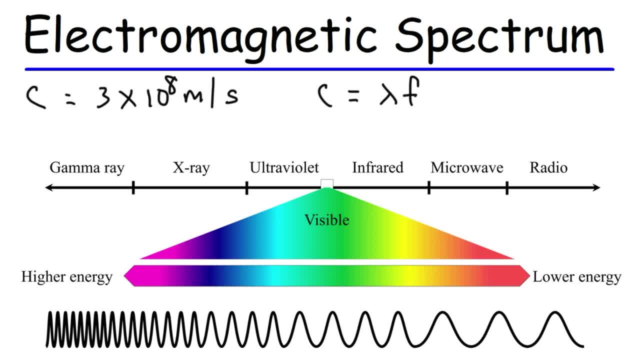 electromagnetic wave is equal to the wavelength times the frequency. What you need to know is that as you move towards the right, that is, towards the radio waves, the wavelength increases. Radio waves have the longest wavelength out of all the electromagnetic radiation in the spectrum. As you go towards the left, the 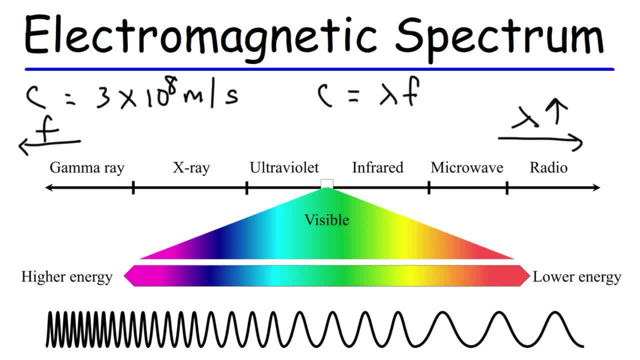 frequency increases, So gamma radiation has the highest frequencies. X-rays, for instance, are higher in frequency than ultraviolet radiation. Microwaves have greater frequency than radio waves. Now, as the frequency increases, the energy increases as well. Gamma rays have more energy than photons that are x-rays, Ultraviolet. 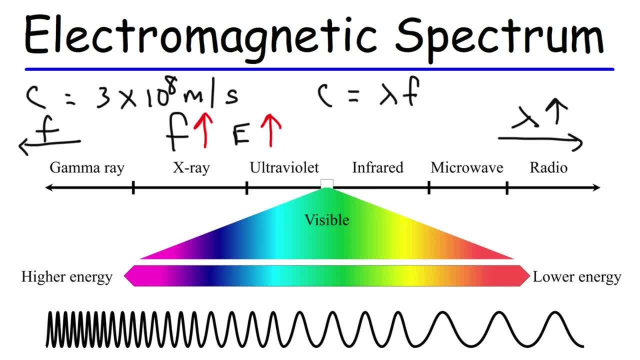 radiation has more energy than visible light, So you need to be able to compare these different forms of radiation in terms of their wavelength, energy and frequency. The energy of a photon is equal to Planck's constant times, the frequency Now Planck's. 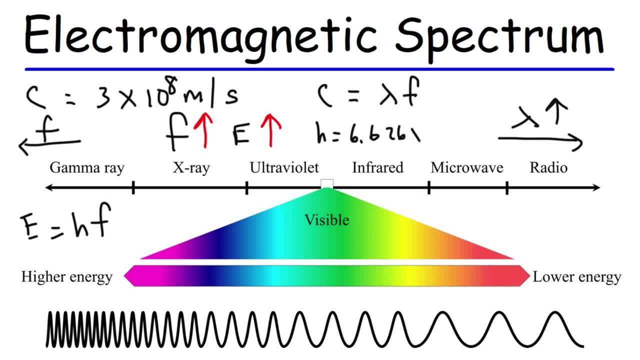 constant is 6.626 times 10 to the negative 34 joules times seconds. So this equation shows that the energy of a photon is directly proportional to its frequency. So as the frequency goes up, the energy of the photon is goes up as well. but now let's work on some practice problems. 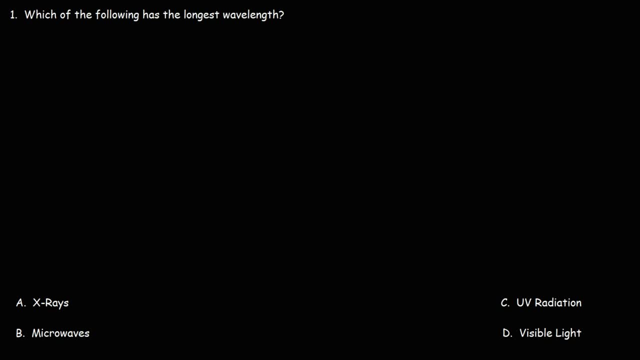 number one. which of the following has the longest wavelength? is it x-rays, microwaves, uv radiation or visible light? what would you say now? i'd like to remember the previous chart, but in a reverse way: first we have radio waves and then come microwaves. 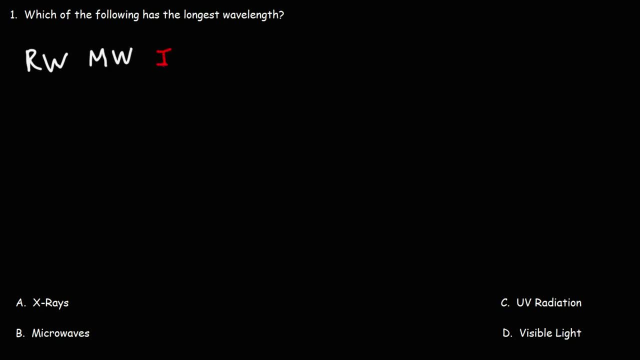 after that it's infrared. after infrared we have visible light, raw gbiv, so it's red light, then it's orange and then yellow and then green light, blue light and then yellow, and then we have violet and after violet is ultraviolet, but this ends visible light. we can't see ultraviolet radiation. 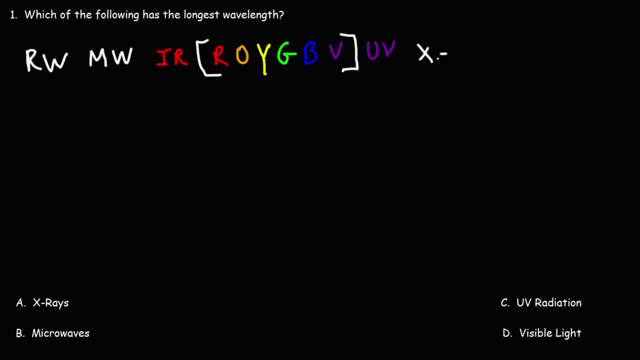 after uv radiation we have x-rays and then gamma radiation. now, remember, radio waves has the longest wavelength. wavelength increases towards radio waves. gamma rays has the highest frequency and it also has the highest energy, so energy and frequency increases towards gamma radiation. so, looking at the options that we have were comparing microwave radiation. 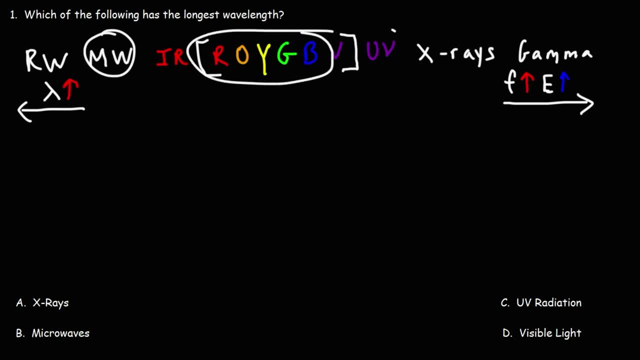 visible light, UV radiation and x-rays. So look for the longest wavelength. That's going to be the one towards the left. Therefore it's microwave radiation. So the correct answer is answer choice B. Now let's move on to number two. 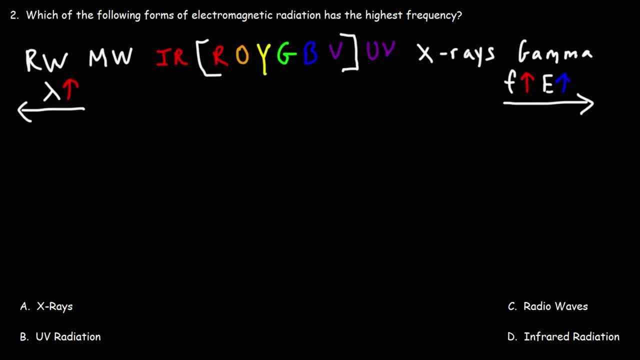 Which of the following forms of electromagnetic radiation has the highest frequency? Is it x-rays, UV radiation, radio waves or infrared radiation? So let's highlight all the options that we're looking at or that's under comparison. So we have infrared radiation, UV radiation, x-rays and radio waves. 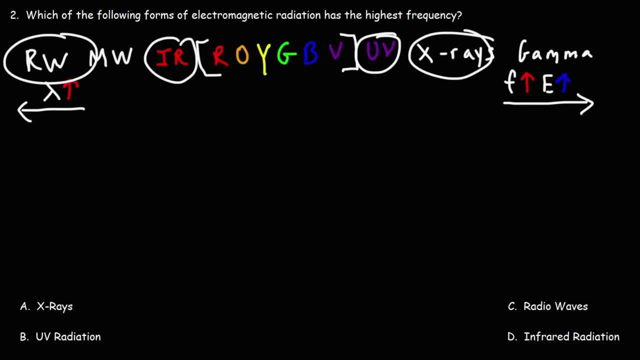 Out of these four, which one has the highest frequency? It's going to be the one closest to the right. So the one with the highest frequency out of what's listed here is x-rays. So the correct answer choice is answer choice A. 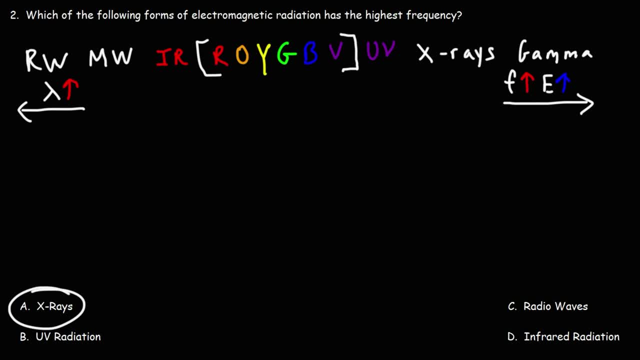 X-rays has the highest frequency of the options listed. Number three: Which of the following colors of visible light has the highest energy? Red light, blue light, yellow light or green light? So let's circle our options. We have red, yellow, green or blue. 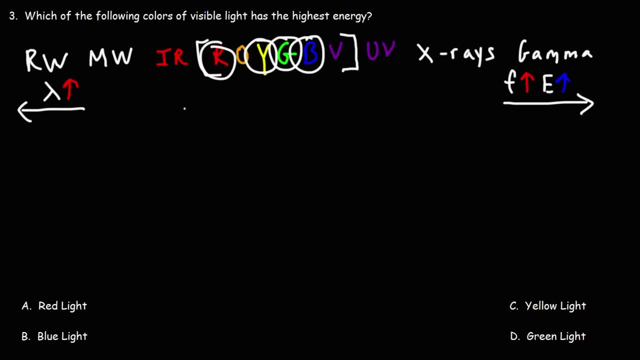 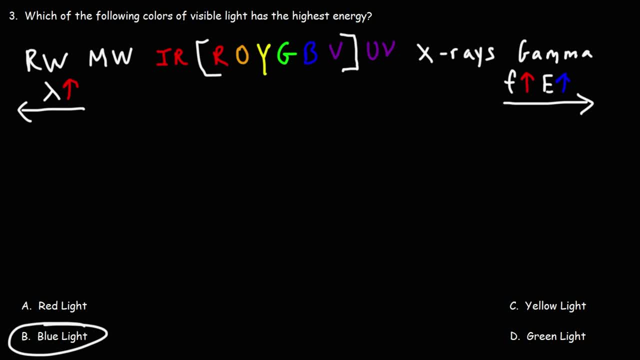 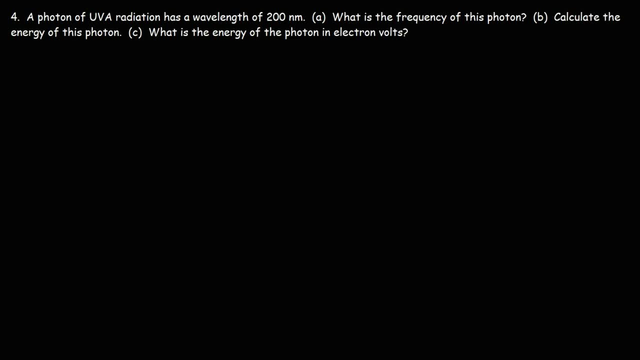 Now let's try number four. A photon of UVA radiation has a wavelength of 200 nanometers. What is the frequency of this photon? So how can we calculate frequency, given wavelength? We know that the speed of light is equal to the 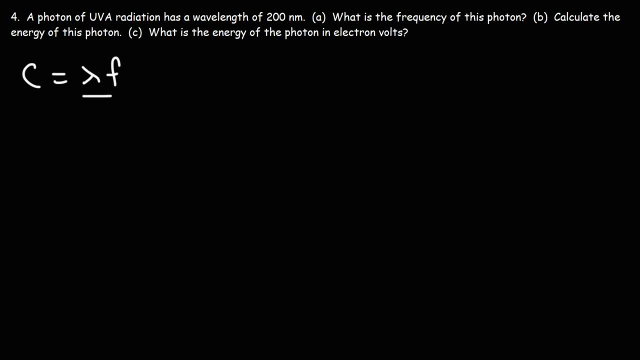 wavelength times the frequency. So to get the frequency we need to divide by lambda. The frequency is going to be equal to the speed of light divided by the wavelength. So we could use that formula for part a. The speed of light is 3 times 10 to the 8 meters per second, and the wavelength of this particular 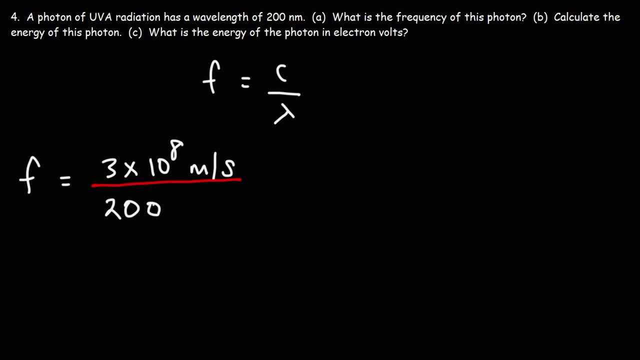 photon of UVA radiation is 200 nanometers. We can write that as 200 times 10 to the negative 9 meters. We could cancel the unit meters and let's plug this in the calculator. so it's true 3 times 10 to the 8, divided by 200 times 10 to negative 9.. 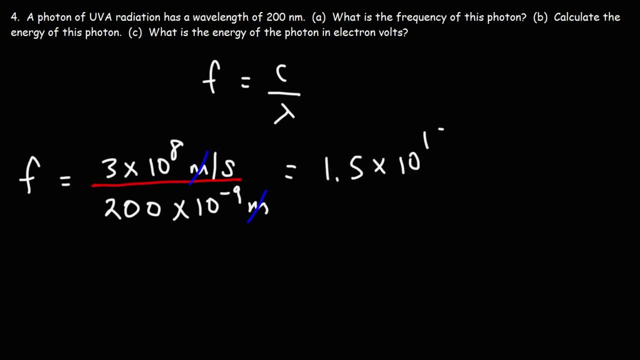 And this is going to be 1.5 times 10 to the 15 hertz, or 1 over seconds. So that's how we can calculate the frequency of this photon. Now let's calculate the energy. The energy of the photon is going to be Planck's constant times: the frequency.